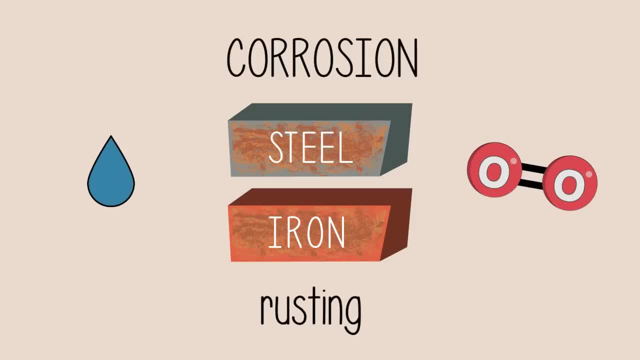 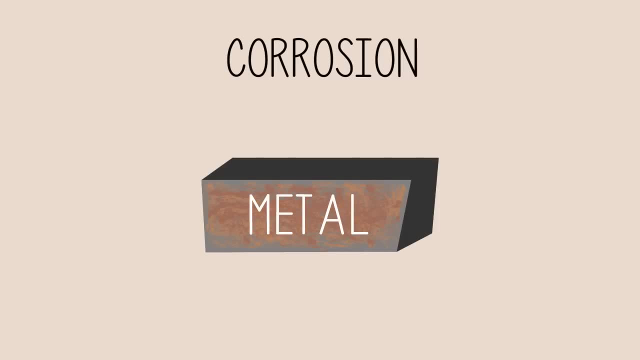 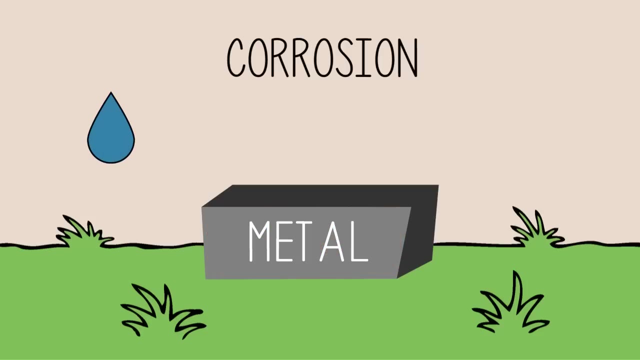 rusting will occur. Rusting describes the corrosion of iron and steel. The term corrosion is used to describe the breakdown of a metal when exposed to the environment. When we say a metal corrodes, we mean that it has reacted with water and oxygen from the environment to form their 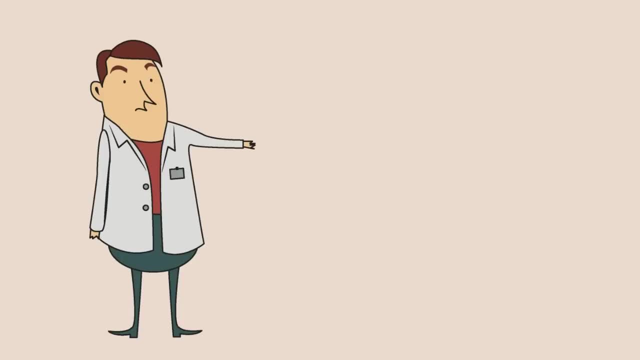 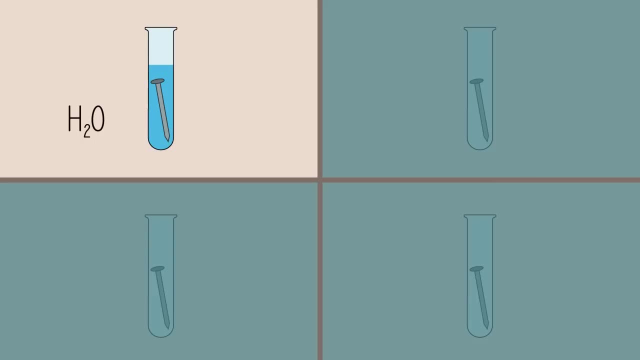 respective oxides. We can demonstrate this using a simple experiment. Place an iron nail in four test tubes. Fill one with regular tap water until the nail is submerged. Fill another with regular tap water and add half a spoonful of sodium chloride. regular table salt. Shake from side. 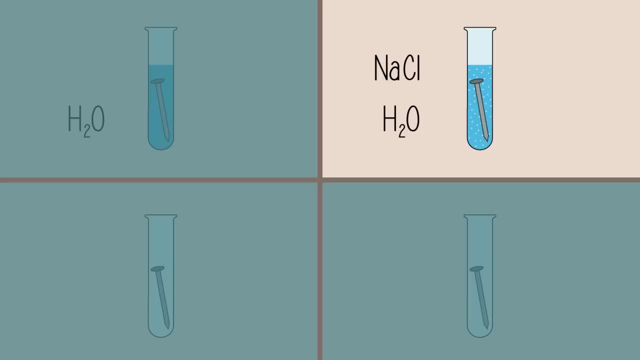 to side. to ensure that sodium chloride fully dissolves, Fill the third test tube with recently boiled water and add a thin layer of oil. When we boil the water, we remove any dissolved oxygen and the layer of oil prevents any oxygen from further dissolving. In the last test tube, add a. 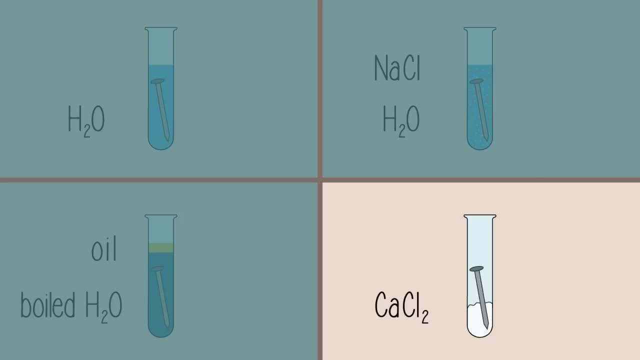 spoonful of calcium chloride. Calcium chloride removes moisture or water. So in the first test tube the nail is exposed to oxygen and moisture. In the second test tube the nail is exposed to oxygen, moisture and salt. So in the third test tube the nail is only exposed to water. In the 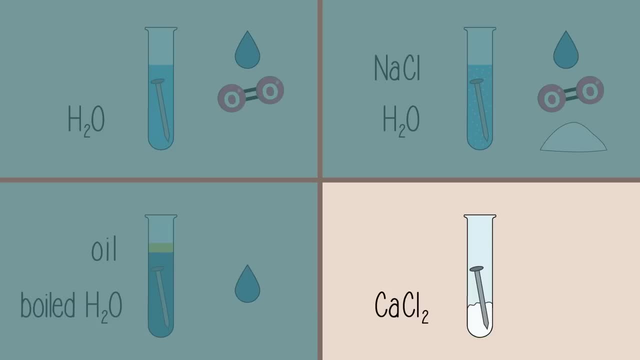 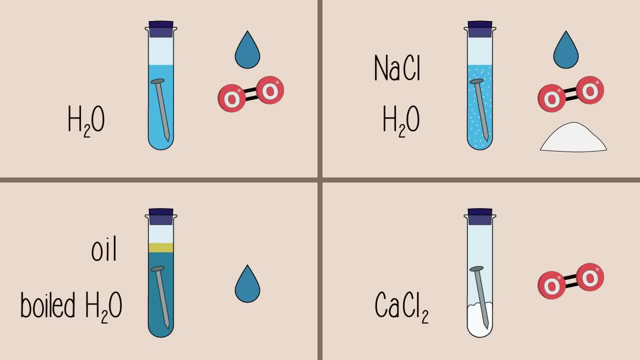 fourth test tube, the nail is exposed only to oxygen. Stopper all four test tubes with a rubber bung and let stand for a couple of days. You will find that the nails in the first and second test tubes have rusted. In particular, the nail in the second test tube has rusted more than the. 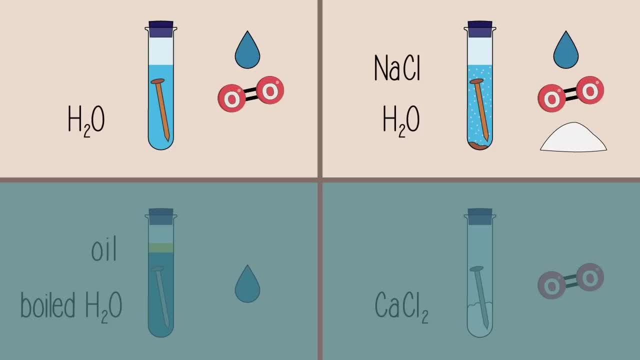 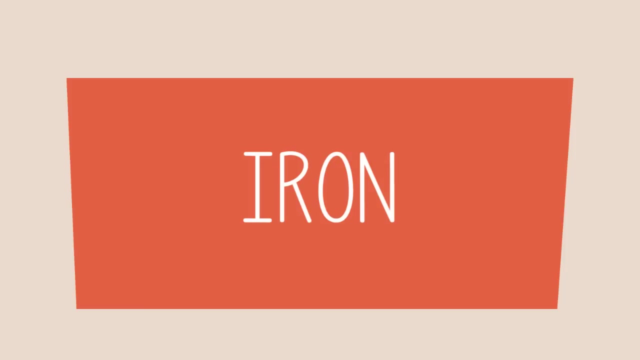 first test tube and the rust has likely flaked off. You may see a reddish brown precipitate at the bottom of these tubes. The nails in the third and fourth test tubes have not rusted. So what has happened here? The iron has undergone an oxidation reaction, forming hydrated iron.